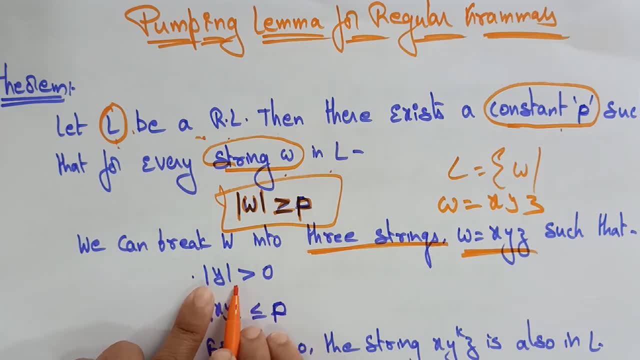 lemma Here the mod Y, that's a positive number. mod Y should be greater than zero. okay, this should be greater than zero. And mod XY is less than or equal to P. means this time this side is less than or equal to P. in on the greater than or equal to P. Okay here, length. 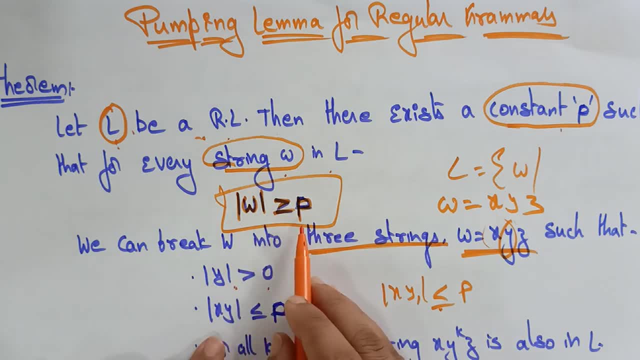 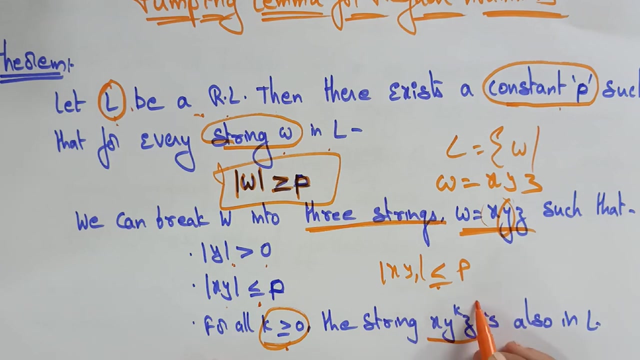 complete the length of the string that W is greater than or equal to P. but here the mod XY is should less than or equal to P. and the third condition is for all K greater than or equal to 0 means I am taking one constant that is greater than or equal to 0, means above 0. then the string X, that is a 3, X, Y, power, K, Z is also in. 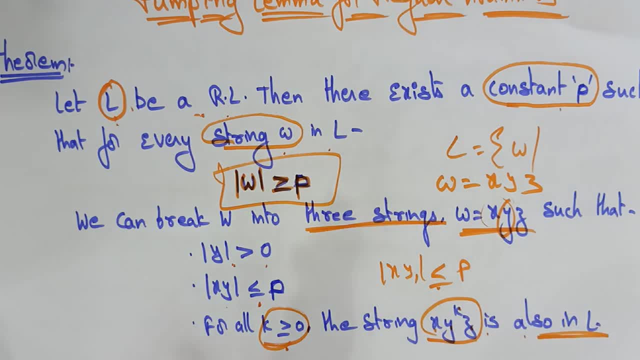 language L. So this is the theorem. it's a theorem of the pumping lemma. It's a simple thing. by seeing this you won't confused. Let's take a concept. if I take in a language L that is a regular language, in that language I am having a constant P, okay, and such that for every string, 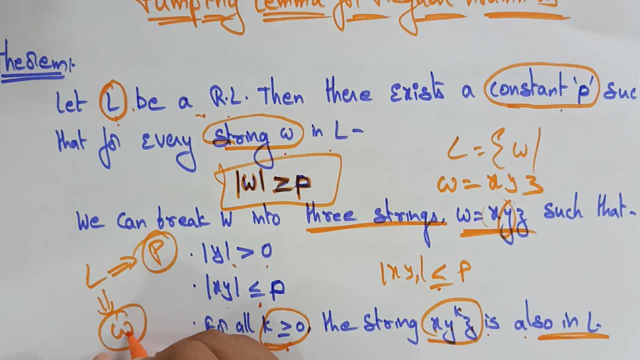 W here in the language you are having a string W in W also, you are having the P right, So that should be: mod W is greater than or equal to this constant. it should be greater than or equal to the constant and we are breaking this into three strings: X, Y, Z, such, 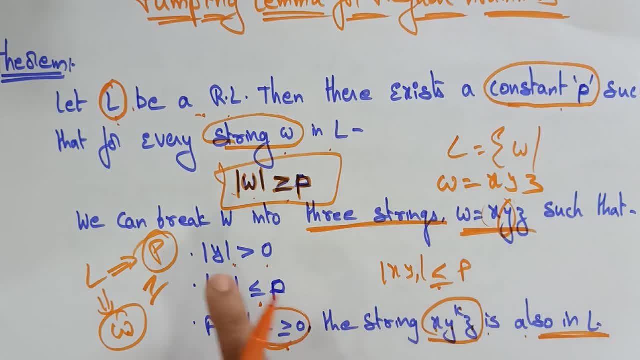 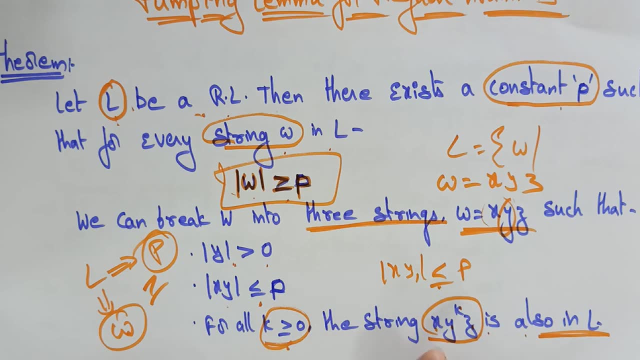 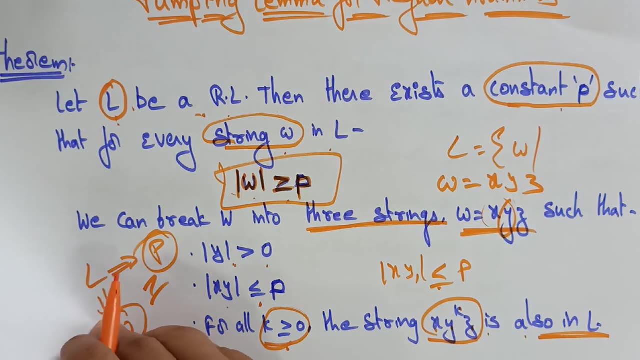 That. what is the condition on these three strings? mod Y should be greater than 0, mod XY should be less than or equal to P and for all K greater than or equal to 0. the string X, Y, power, K, Z is also in language, So let's see the proof, then you will understand. before going to that, let me explain. 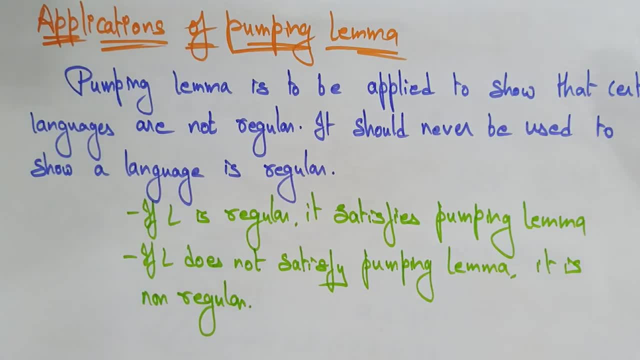 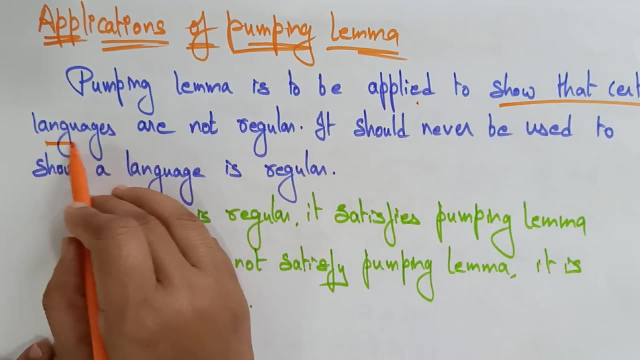 what are the different applications of the pumping lemma, Actually, why we are using this pumping lemma? what is the use of the pumping lemma? The pumping lemma is to be applied To show that certain languages are not regular. This what is going to do. it is going to do. it is. 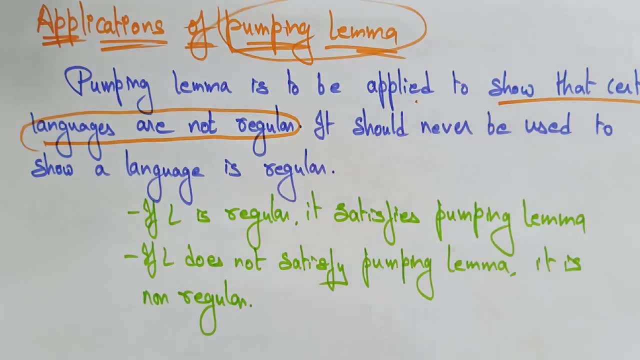 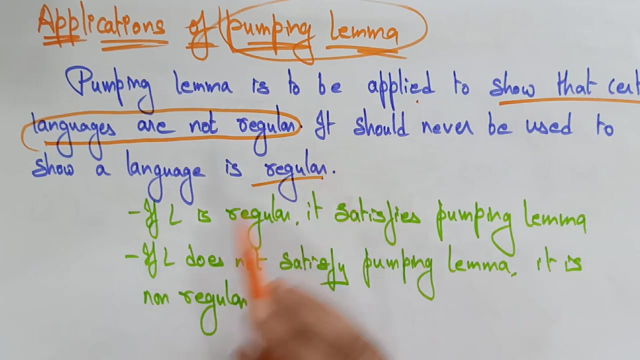 going to prove that some languages are not regular. okay, What is the use of pumping lemma means you have to say that pumping lemma is used to apply to show that certain languages are not regular and it should never be used to show a language is regular, So you don't show this language is. 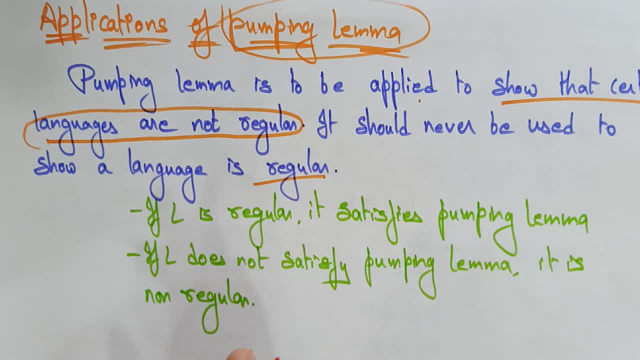 regular. You always take the contradiction: Show that certain languages are not regular, okay, Regular language means no need to take that. if it is regular, okay, leave it. So for some languages you have to show that they are not regular. In that cases you go for the pumping lemma. So if L is regular, it satisfies a pumping lemma, then no need. 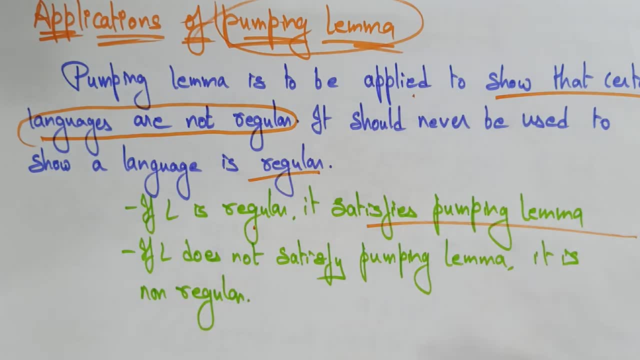 to you can't do anything. okay, It's already like regular. it satisfies a pumping lemma. If L does not satisfy pumping lemma, then it is not regular. Okay, so the thing is, the pumping lemma is applied to show that certain languages are not regular. 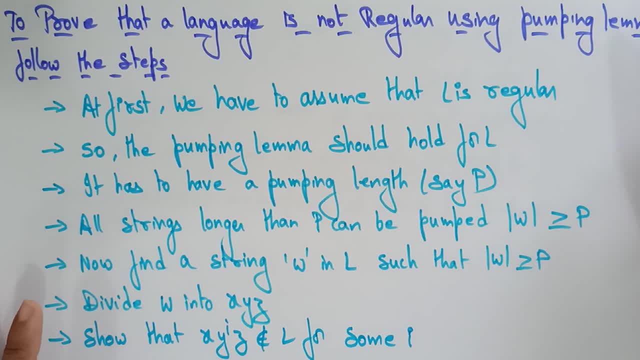 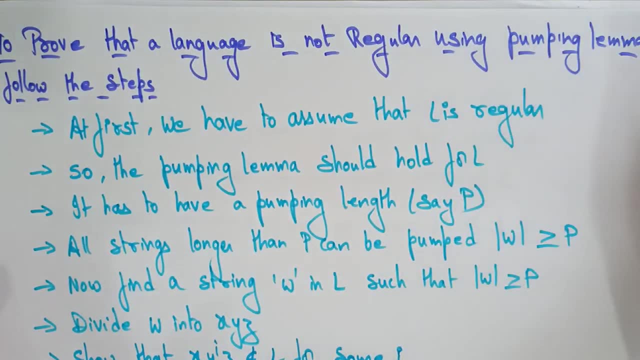 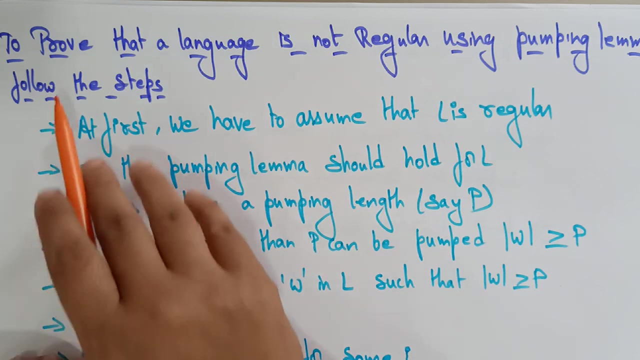 Let me take the steps that are involved in the pumping lemma. So if you see these steps then you can be clearly understood. To prove that I hear the, whatever the theorem I have taken, I am proving for here the language that should not be a regular, that I have to be proved that, not regular, To prove 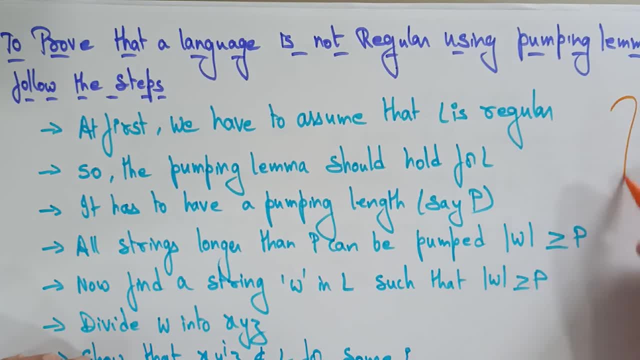 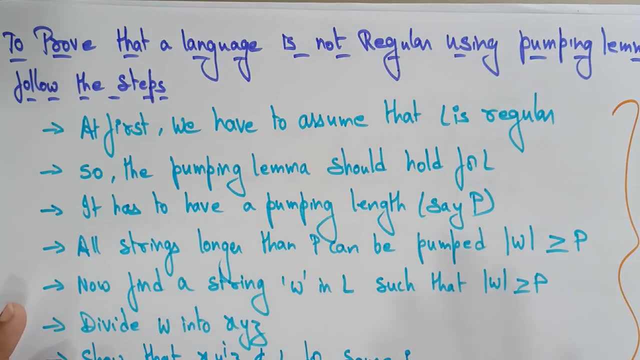 that a language is not regular using pumping lemma. we have to follow these steps. If you follow these steps, you can see that the language is not regular by using pumping lemma. And first we have to assume L is a regular. So starting you take the contradiction. Let's assume, whatever the language, that I have taken. 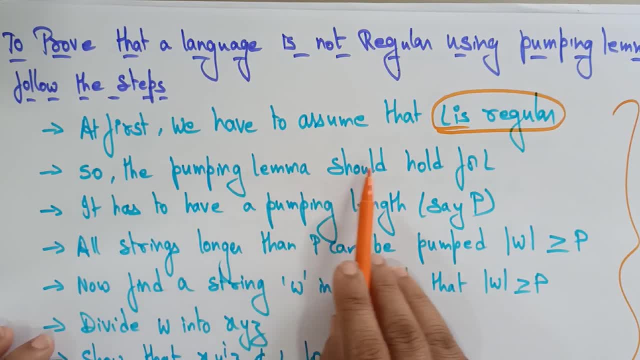 it is a regular Next. so the pumping lemma should hold this language L. Okay, now this pumping lemma is holding this language L. So whatever the length it should be holding the length L, It has to have a pumping length, say P. I said some constant has to be present, So it has to have a pumping length, say P. 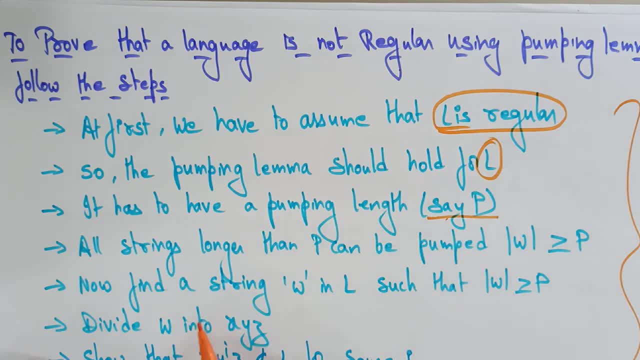 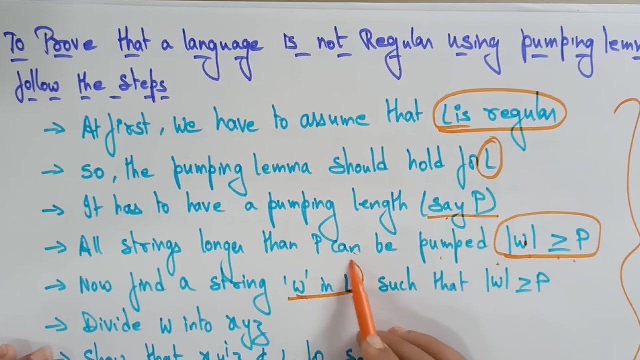 Okay, that is a pumping length, say P, And all strings longer than P can be pumped to. that is mod W greater than or equal to P. That we know that. Now find a string W. So now I need to find a string W in L which is present in L, such that mod P should greater than or equal to P. So whatever the string, 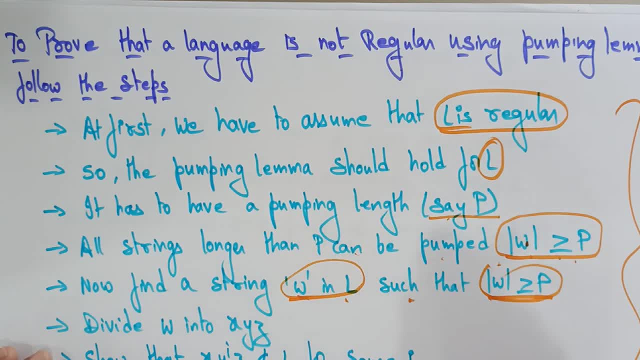 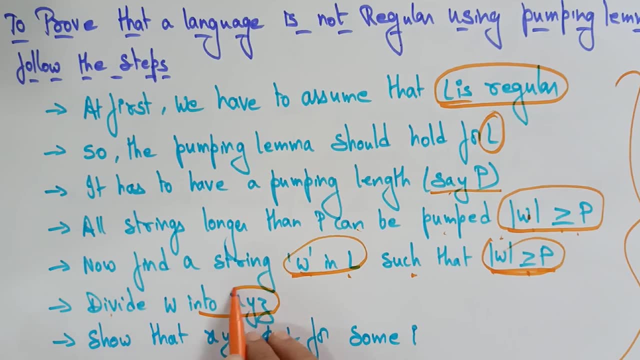 that you are going to find out, in the language L that should be greater than or equal to P, That you have to be remember that. So after finding the string, you have to divide it into X, Y, Z. So whatever the string that you got,